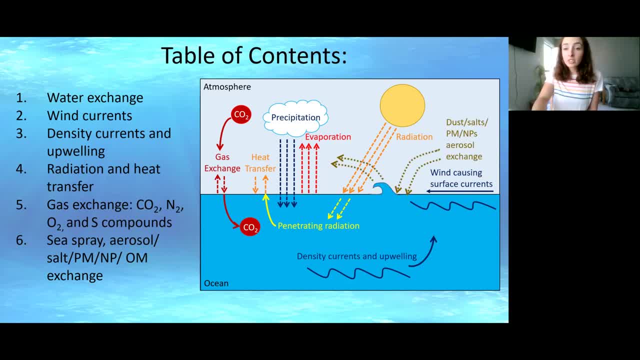 well as other things- Those are the main ones I'll be hitting- And aerosol exchange through atmosphere to ocean interactions, as well as sea spray, ocean to atmosphere interactions, And so we'll be talking about all of these in today's video, in this order, So starting with precipitation. 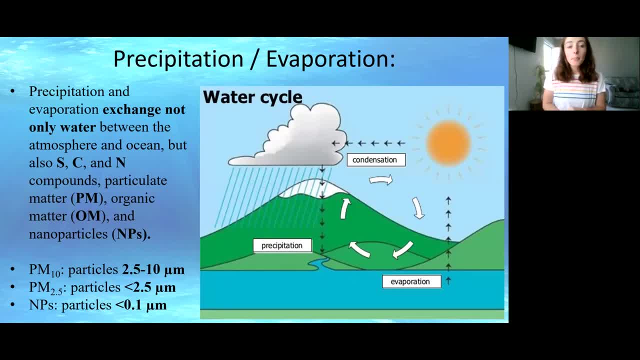 and evaporation. this one seems like a pretty simple one, but when we're talking about water exchange through precipitation and evaporation, this isn't only exchanging water. It's actually exchanging much more, because water can actually carry with it constituents from the atmosphere to the ocean or from the ocean to the atmosphere through evaporation. So this is a 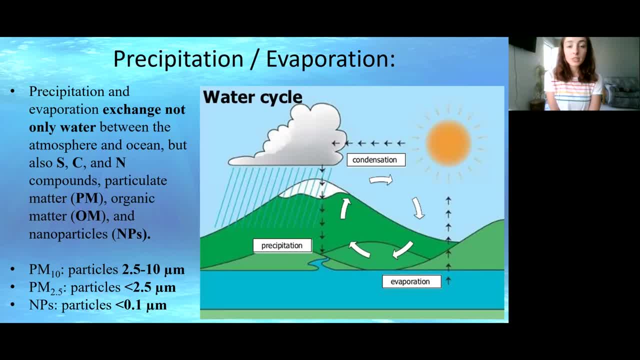 cycle. that is hugely important for the water cycle as a whole, but also for cycling other elements, as well as other particles, or particulate matter, abbreviated PM, or organic matter, OM, or nanoparticles or NPs, And we'll be talking about all of these in much more detail in the pollution. 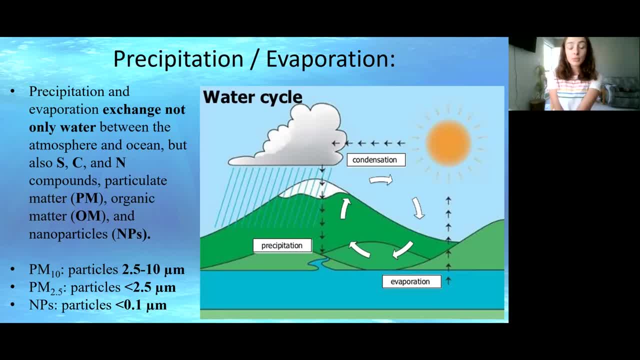 episode, because when in the afternoon we're going to be talking about all of these in much more detail in the pollution episode, because when in the afternoon we're going to be talking about: wow, these can be harmful pollutants. But basically just to introduce the concept PM or particulate, 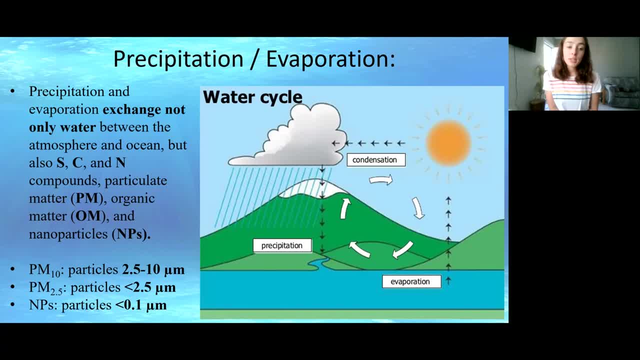 matter has two main categories: either PM 10 or PM 2.5, that just has to do with the size of particulates, And so when the particles are 2.52 microns or micrometers, then it's PM 10.. If it's, 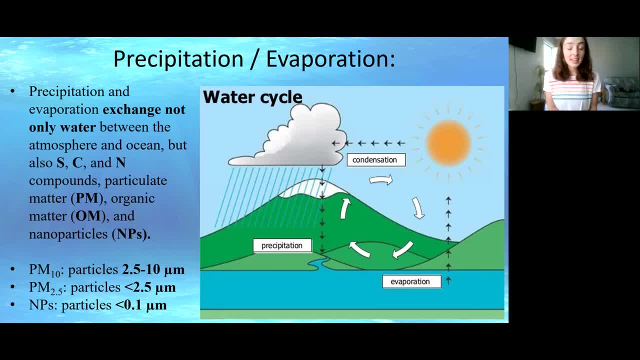 less than 2.5 microns, then it's PM 2.5.. And if it's less than 0.1 microns, this is really tiny, it's a nanoparticle. So, and we're going to be talking about how molecules can change the 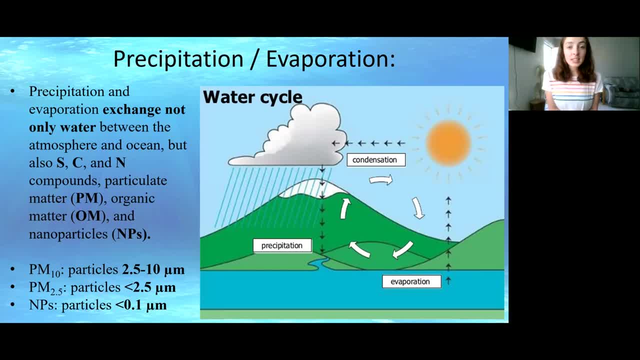 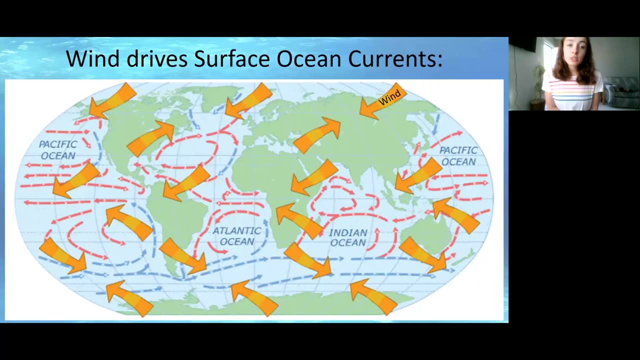 All of these contribute a lot to pollution and our health, as well as earth processes as a whole, climate, weather, etc. So it's just important to remember that these things can be transported by water through evaporation and precipitation. So we'll come back to those later, but first we need to just introduce the concept that wind drives surface currents in the ocean. 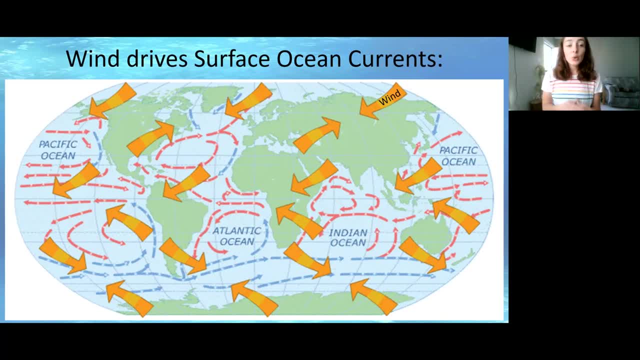 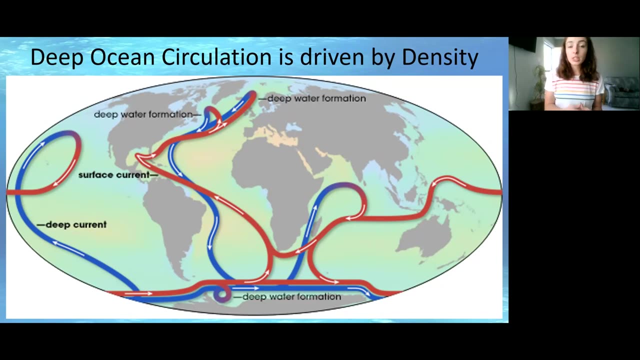 These orange arrows are showing atmospheric winds, and the red and blue arrows are showing oceanic circulations, And so wind plays a huge role. Another thing, though, that plays a huge role in ocean circulation is density, So the density of the water can also really affect the circulation, and the density of the water changes depending on salinity or salt content and temperature. 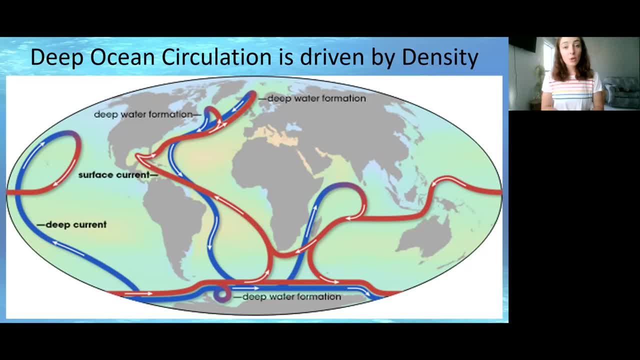 So this is called thermohaline circulation- and I'll be talking about this in a different episode- as well as atmospheric circulations. So that's just to get out of the way to understand that that's another way that the ocean and the atmosphere can interact. 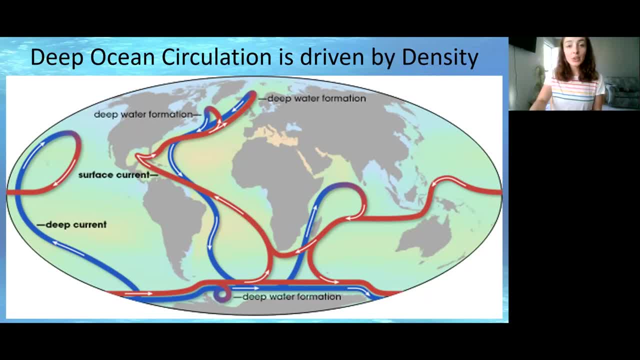 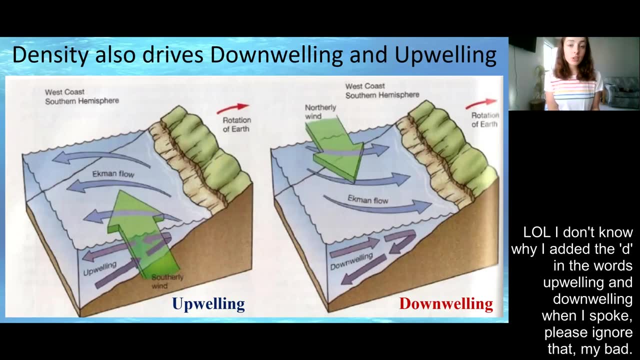 But now we're going to move on to the other points I was going to make in this video. The next thing is also having to do with density, but it's down-dwelling and up-dwelling in the ocean, And so this typically occurs because, as the circulation of the ocean comes to an edge, a continental edge, 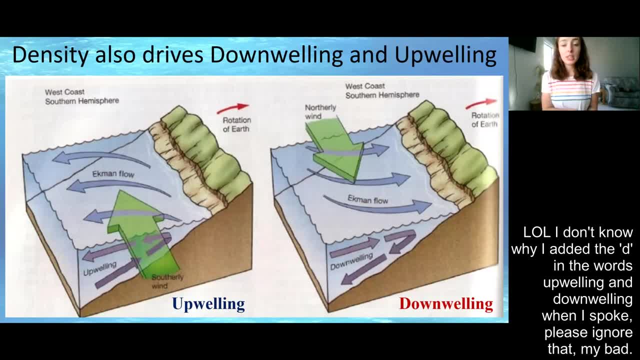 it will, depending on the wind direction and the surface current direction, either up-dwell or down-dwell, meaning that bottom waters that are typically separated from the upper waters because of density separation will come up or up-well up into the surface. 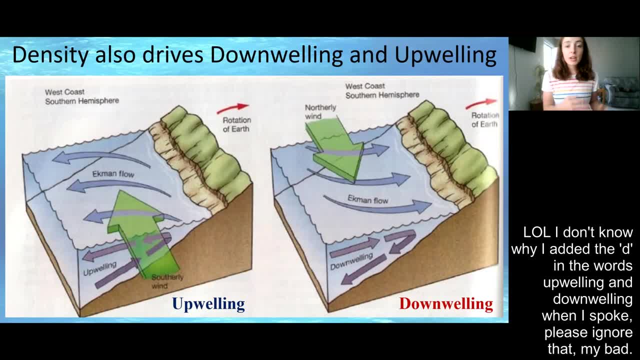 And so this is where we're going to be talking about down-dwelling and surface waters, whereas down-dwelling is just the opposite process. Surface waters, or more fresh oxygenated waters will go down and introduce more fresh and oxygenated waters to those saline, anoxic bottom waters. 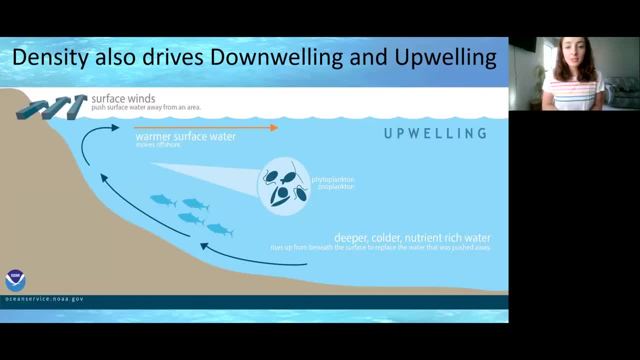 And the importance of these processes are in continental shelf environments and ecosystems. So what up-dwelling and down-dwelling- any of the mixing- really does is, for example, during up-dwelling, deeper nutrient-rich waters will come up to the surface and provide nutrients. 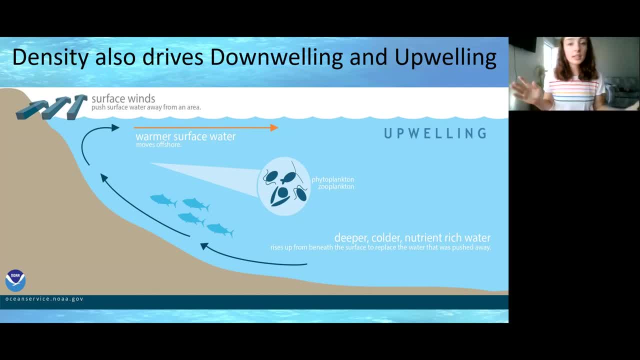 And this will create a bunch of biodiversity in an area where up-dwelling and down-dwelling occurs often, because this mixing just really makes the water very nutrient-rich, well-oxygenated and just more primed to hold life. So this is why up-dwelling and down-dwelling are really important. 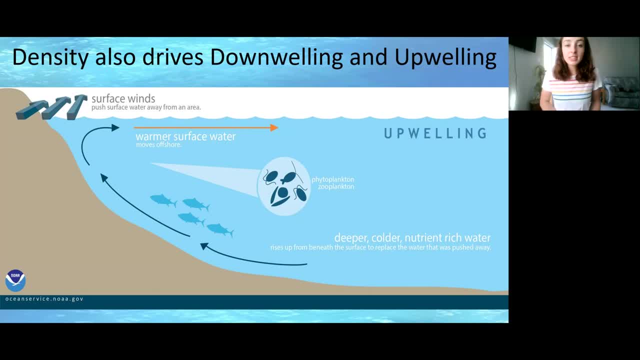 And when continental margins are rich in biodiversity in their surface waters of the ocean, then this can cause an atmospheric effect because there's more photosynthesis occurring there, There's more oxygen going into the ocean, There's more carbon dioxide being pumped into the ocean. 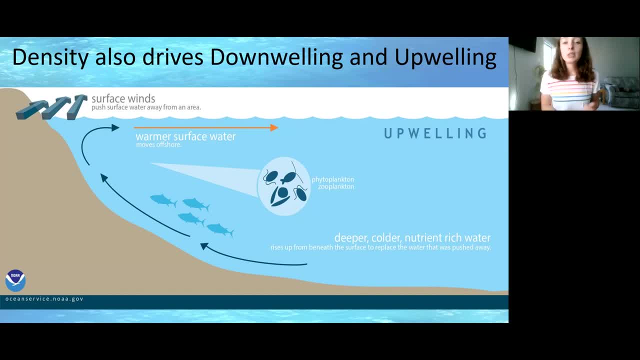 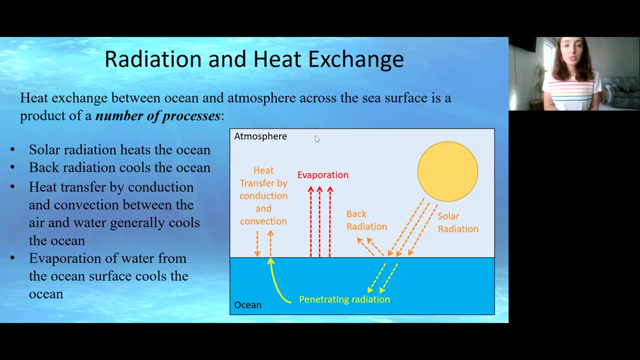 And so these up-dwelling and down-dwelling events don't only have to affect the ocean and the ocean's biodiversity, They can also affect the atmosphere as well as the terrestrial biodiversity along that coast. Next, radiation and heat transfer. Heat can actually be exchanged between the ocean and atmosphere through a number of different processes. 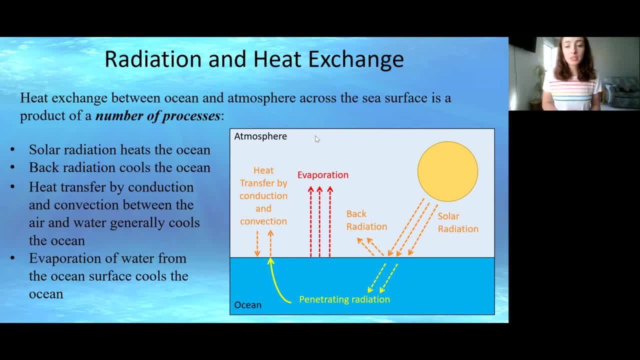 But they all kind of play a role back to each other so they're connected. But basically solar radiation or air or light from the sun can be absorbed by the ocean or reflected in back radiation from the ocean which can either heat or cool the ocean respectively. 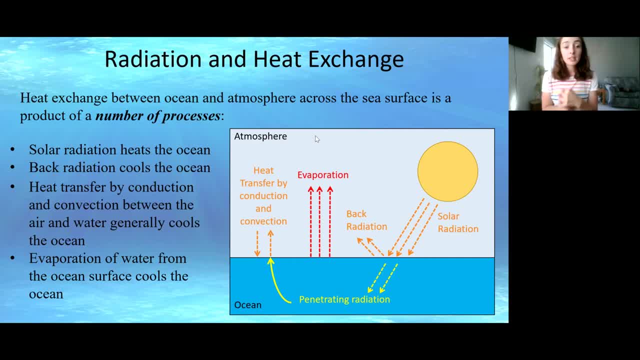 Another thing is heat transfer by conduction and convection between the air and water, which generally can cool the ocean as well, And evaporation can also cool the ocean. Now a lot of these seem like they're cooling the ocean, but the ocean's not going to really lose all its heat. 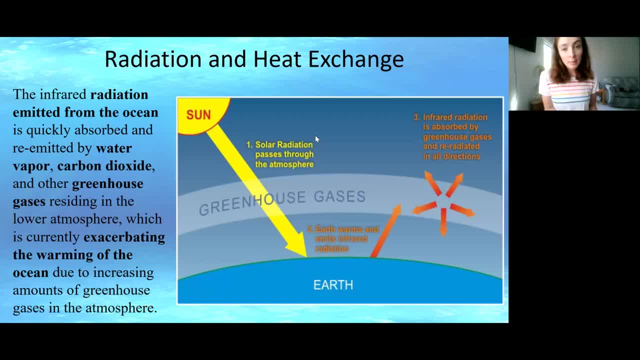 And that's because processes like the greenhouse effect can trap heat and continually warm the ocean. And so what happens? The back? radiation emitted from the ocean can quickly be absorbed and re-emitted by water vapor, carbon dioxide and other greenhouse gases in the lower atmosphere above the ocean, and then be reabsorbed by the ocean. 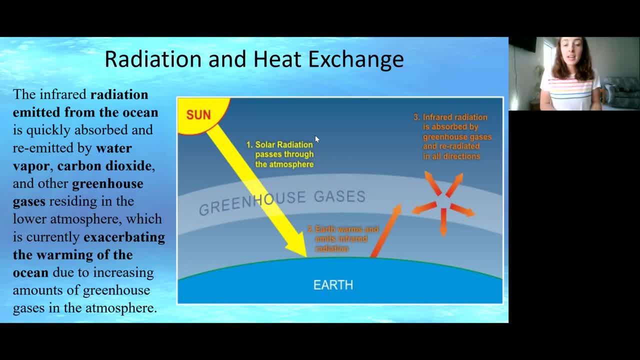 And this is a good, naturally occurring effect and keeps the ocean warm from losing all its heat in a normal climate regime. But currently we're kind of putting this out of balance. So instead of cooling and heating and a balancing act, the ocean is currently warming because 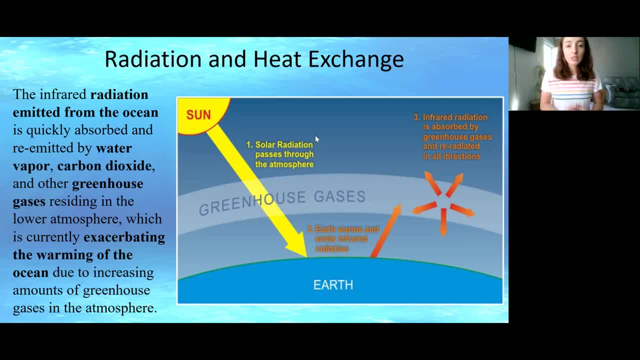 The ocean is currently warming. because The ocean is currently warming because we're exacerbating this greenhouse effect, causing the cooling of the ocean to be out of balance with the heating of the ocean, and the ocean's getting more heat than it is cooling, And so this greenhouse 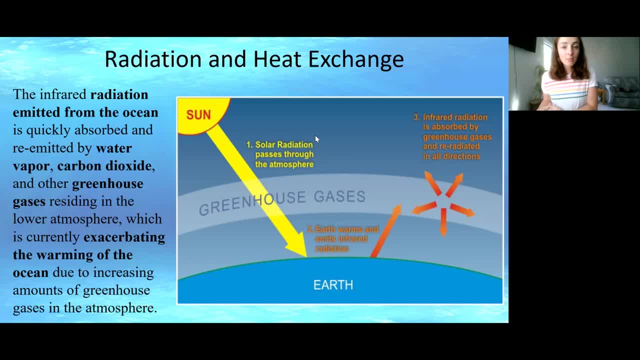 effect, although we currently associate it with a really negative meaning, isn't necessarily bad, and it doesn't always have to be anthropogenic. It can be natural and it can be good, because we do want some heat on Earth. We want to balance, But this balancing act is currently being put out of. 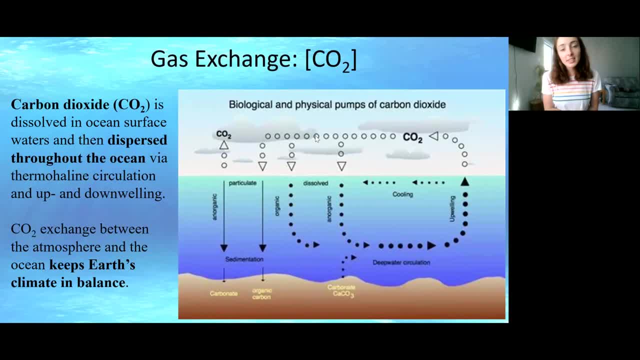 balance, and so that's when the greenhouse effect gets dangerous. And now getting to gas exchange. first we'll talk about carbon dioxide, because why not? more bad news, right? But basically carbon dioxide can be exchanged from the atmosphere to the ocean and vice versa. 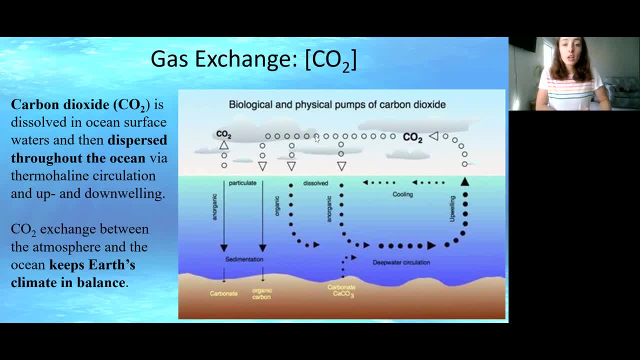 And when the carbon dioxide is dissolved in the ocean, it becomes carbonic acid, which can break down into bicarbonate and carbonate ions, which I talked about in the ocean acidification video. But basically it's acidifying the oceans because it's increasing the hydrogen ion content of the 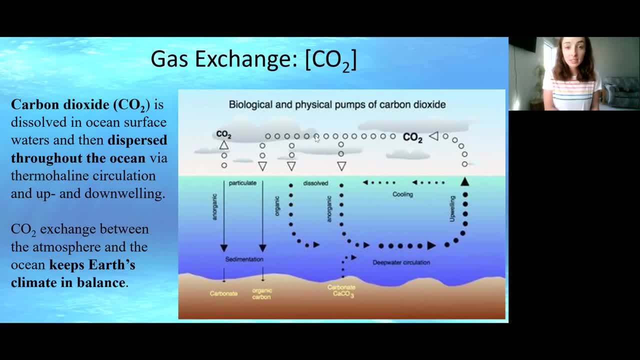 oceans, and this is really not good for the calcium carbonate Organisms you can see here at the bottom of this figure. that's calcium carbonate, basically CaCO3, are organisms that get dissolved in acidic conditions, And so this is really not good. 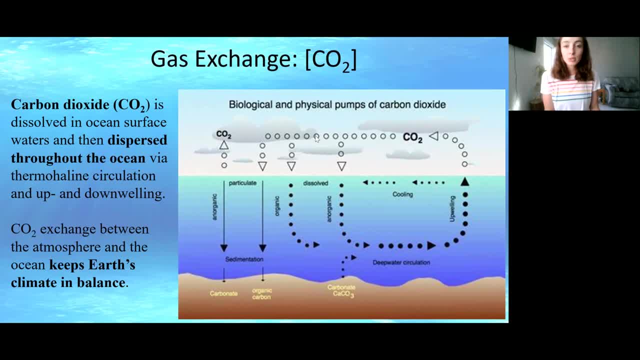 if the ocean is becoming more acidic, We don't want those organisms to all dissolve, because they're a huge deal for life in the ocean, And so if they all dissolve, we're first of all not going to have the huge ecosystems associated with coral reefs, and we're also not going to have that. 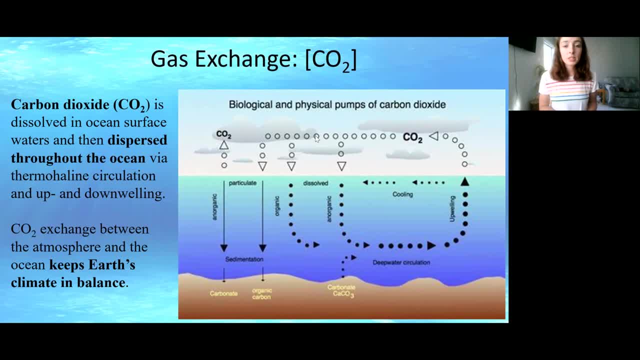 calcium carbonate buffer anymore in the ocean to keep the ocean from accelerating, And so we're not going to have that calcium carbonate buffer anymore in the ocean to keep the ocean from acidifying too fast, And so that would just be really detrimental to all marine life and 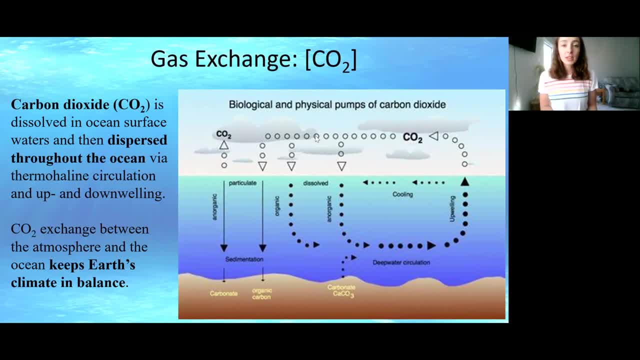 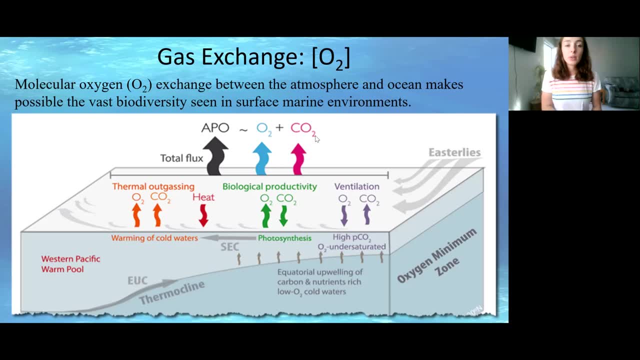 therefore our lives, because the marine ecosystem affects the terrestrial ecosystem in a direct way. So, but if you want more on that, you can watch the ocean acidification video. But now I'm going to move on to oxygen. Oxygen is a major component of our atmosphere and our oceans, as either 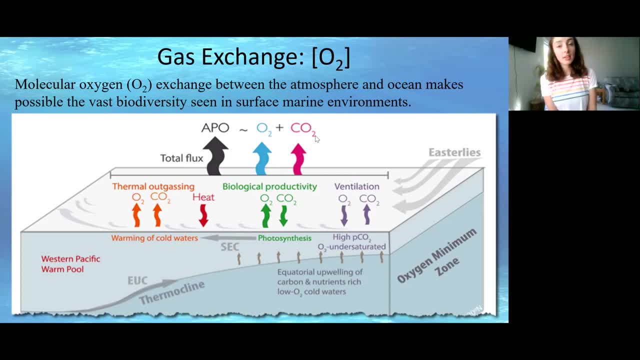 molecular oxygen in the gaseous state or dissolved molecular oxygen in the ocean. And dissolved oxygen in the ocean is really important for marine life And so we're going to have to oxygen. So it is important that this gas gets exchanged from the atmosphere to the ocean and 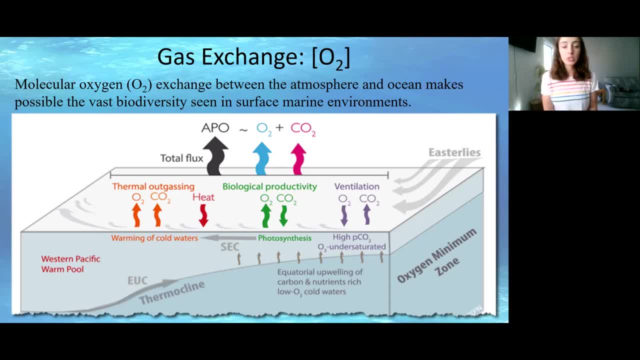 vice versa, And typically what happens with oxygen exchange is that surface waters become really heavily oxygenated and all the photosynthetic activity is occurring there, because the sunlight only penetrates so deep in the water And so those surface waters are really oxygenated And as you go lower in depth in the ocean you're going to have less oxygen. 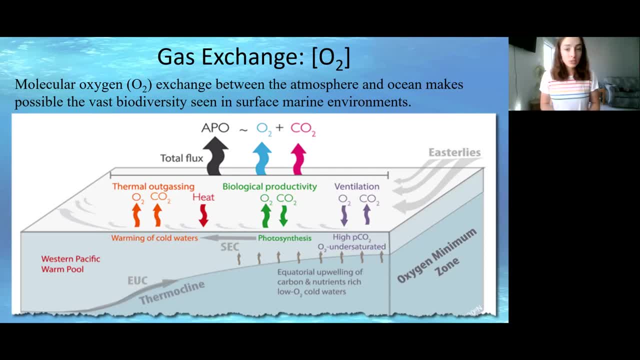 And that's normal to have depleted oxygen with depth, because those deeper, more dense and anoxic or oxygen depleted waters just don't typically mix with the top waters unless you have upwelling or downwelling. However, right now we are causing more oxygen depleted zones in the 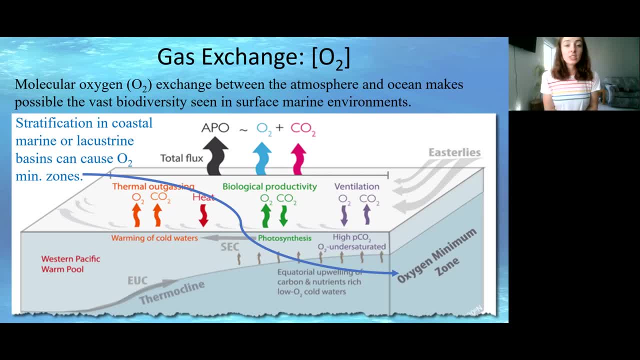 ocean than normal, at an increasingly fast rate, And these can either be called oxygen depletion zones or minimum zones. And so now the question is: is this natural or anthropogenic? Well, oxygen is becoming increasingly depleted in the ocean because of combustion of fossil fuels And 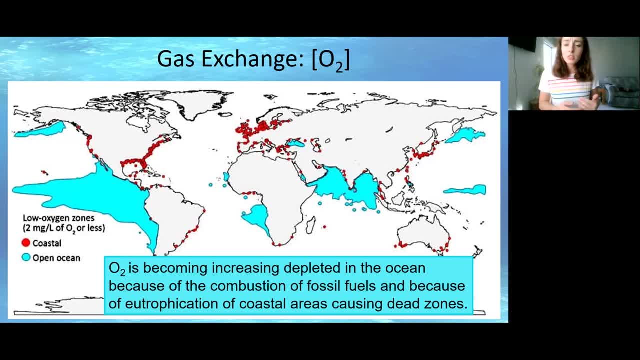 so we're depleting oxygen- The atmosphere- but we're also directly depleting oxygen from the ocean because of eutrophication, which is a fancy word for just over supplying coastal areas with a bunch of nutrients- And I know nutrients is probably a word that you might associate with good things, but really what? this? 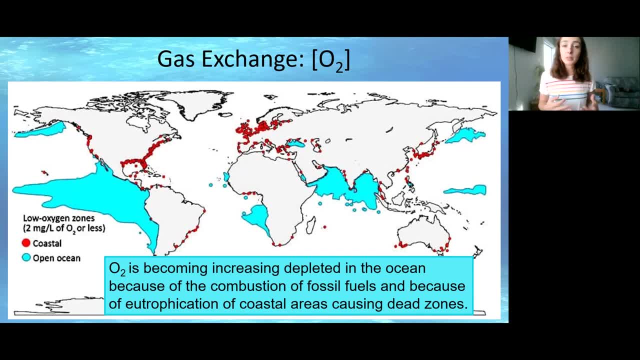 causes is a lot of areas. The Gulf of Mexico is a good example, where the Mississippi river trains into. the Gulf of Mexico is a huge dead zone, which means no oxygen And the reason for this is so many nutrients and pollutants from agricultural processes or whatever it might be. 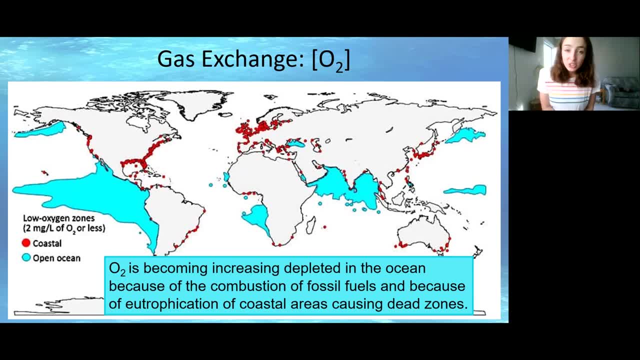 It released into the coastal area right there and causes a sharp increase in primary production and huge algal blooms. And all of this takes up so much oxygen that there's none left over And all that water under the algal blooms is anoxic. 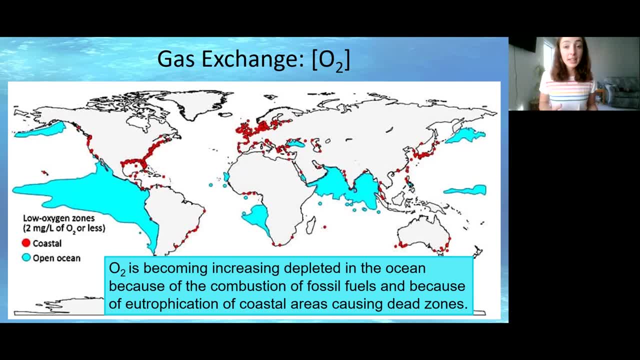 There's no more oxygen, or even yucinic, which just means sulfitic and anoxic, And so very little biodiversity can happen there And you're not typically going to see any life that can actually breathe oxygen there, And so that is all. 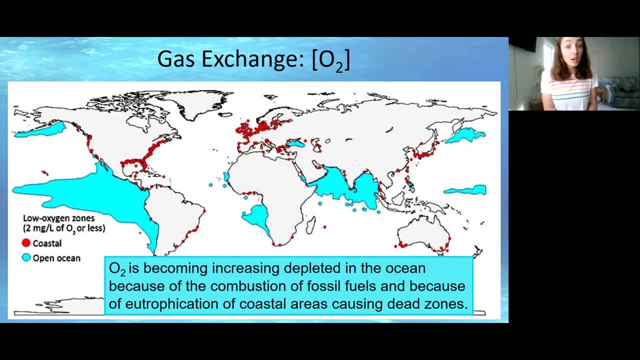 going to die, And that's happening at a rate in which oxygen breathing life in the ocean can't keep up with, at the rates that we're causing their environment to become anoxic, And so they're dying, And that's why we call these dead zones. 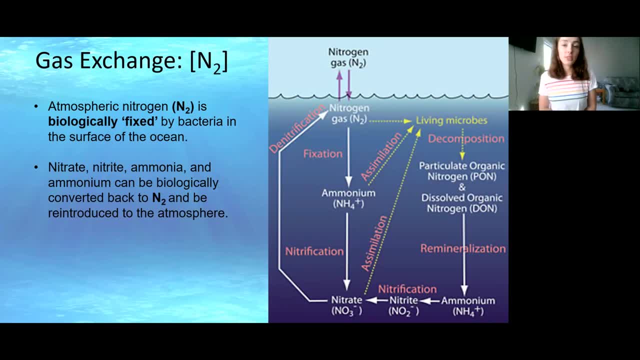 Next, nitrogen exchange. Nitrogen is a huge component of our atmosphere- Around 80% of our atmosphere is nitrogen 2 or nitrogen gas- And this can become exchanged into the ocean And that is where it can be transformed by bacteria that can. 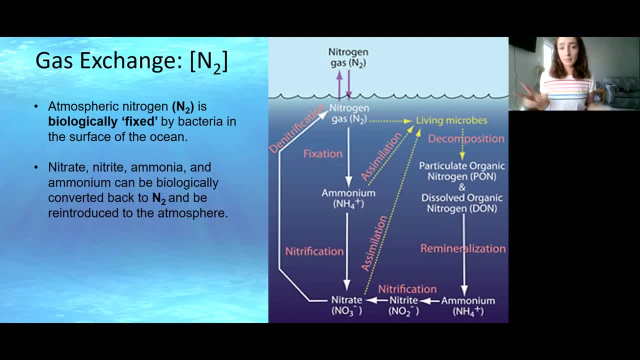 fix it into other compounds like ammonia, which can be nitrified into nitrate or nitrite and then assimilated into microbes, bodies or plants or animals or what have you. And all these processes and all these different compounds of nitrogen can then be. 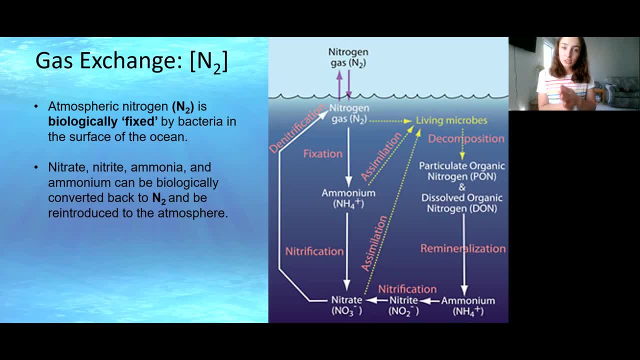 denitrified back into nitrogen 2, atmospheric nitrogen gas and reintroduced into the atmosphere, And this is all a cycle And it's pretty much in balance. Everything that's a little bit off balance right now in terms of nitrogen in the environment is nitrogen oxides and ammonia, And this is 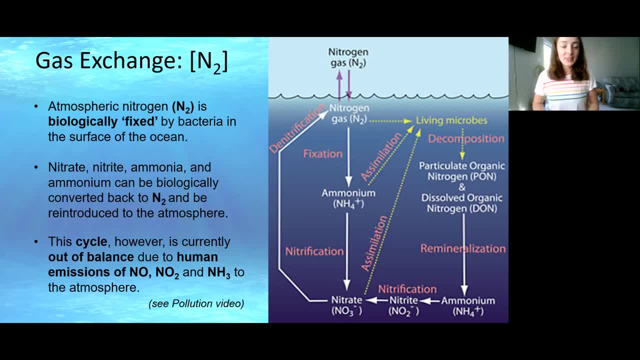 because these are pollutants that we release And so obviously we are kind of putting this cycle out of balance, And so we want to discuss that, And so I discussed that in the pollution video. So if you want more on that, see that video. Next I'm discussing sulfur. 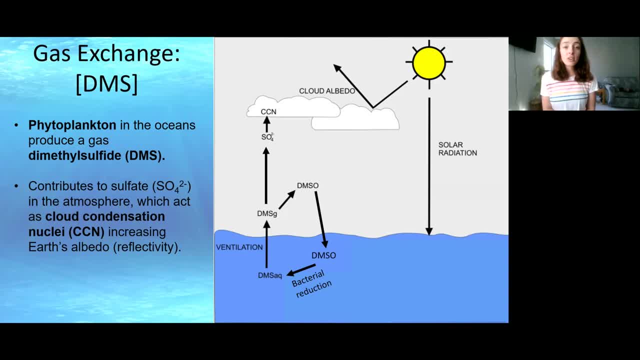 So the main sulfur compound I'll be discussing in this episode is called DMS or dimethyl sulfide, And this compound is important because it's a very important component of the environment. It's a very important component of the environment. It's a very important component of the environment. 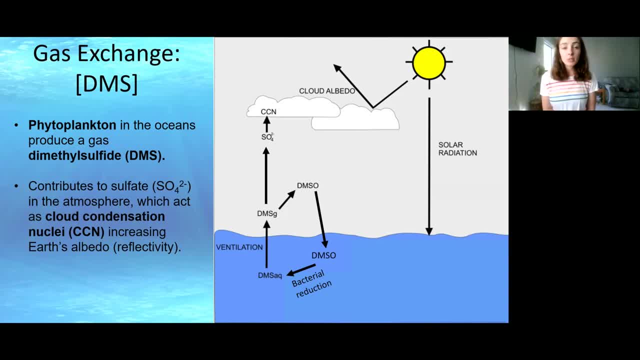 Because in the ocean what happens is organisms- bacteria, whatnot- can use DMSO or dimethyl sulfoxide and reduce it as a way of metabolizing. That's how they live. They take up that and then they produce DMS, And then that can be released into the atmosphere and then oxidized into sulfate particles that can act as cloud. 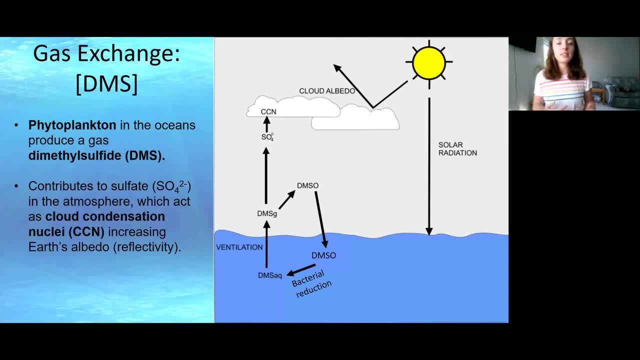 condensation nuclei in the atmosphere. Basically, what that means is that they can act as sites for water droplets to accumulate onto and become clouds, And clouds can act to increase the albedo of Earth, which is really important for fighting climate change, because albedo just means reflectivity of Earth. 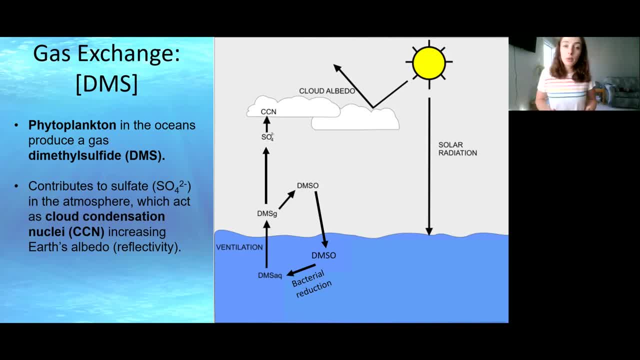 And we really want to reflect all the solar rays that we can, because that will help cool down Earth. Now, this is true, But another bad thing about, say, sulfate in the atmosphere is that sulfur oxide compounds in the atmosphere aren't the best, because they can contribute to acid rain. 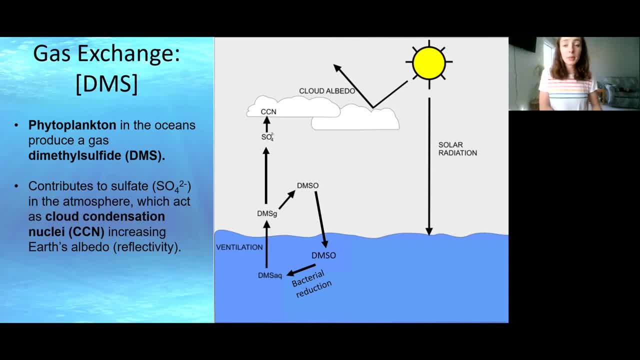 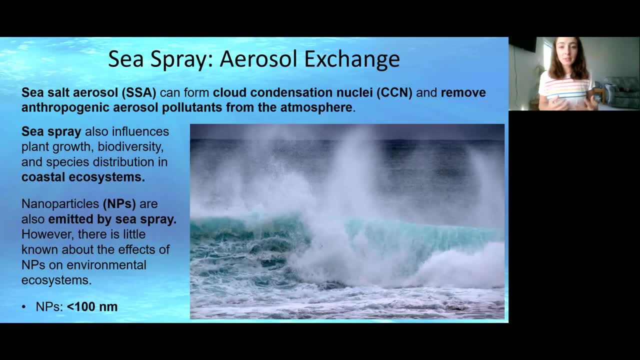 So there are ups and downs to DMS emission from the ocean, But for now we're going to leave it at. it increases our sulfur dioxide, Albedo, and it's good. Next I want to discuss kind of less on gas, more on particles or aerosols. So particles and the air, And examples of these are sea salt emitted from sea spray, which is just waves that crash and all these tiny water droplets can go up into the air and release aerosols. So salts from the ocean or salts from dust, So, like Sahara, dust can transport all throughout the world as well as other desert dust. 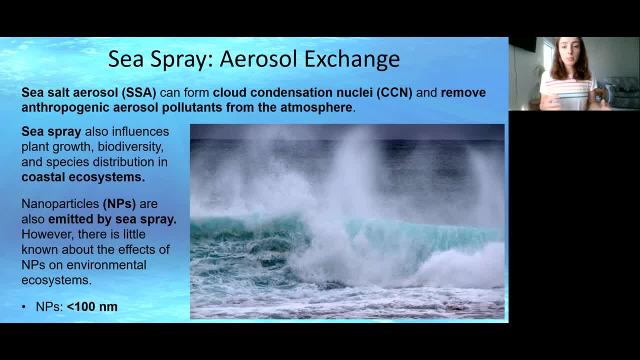 Nanoparticles can either be burned- We use words breaking down from these other aerosols- or can be formed from other natural processes. Nanoparticles can also be formed from manmade processes, But we'll probably talk about that in a different video, But for now just no. sea salts, dust, nanoparticles, particulate matter- We just we discussed at the beginning on the different sizes, basically particles in the air and atmosphere that exchange. All of these are one in the same. They are very complex and they can't really be covered in one side because there's so many different particles that can be exchanged from the atmosphere and ocean and they can't really be. 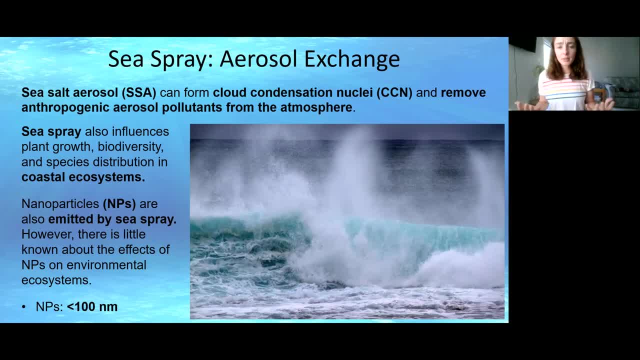 지� biology or師 ORY can't all be discussed as if they behave in the same way. but basically sea salt aerosols typically can be beneficial because they also can act as cloud condensation nuclei and therefore increase our salpito, and they can also remove anthropogenic aerosol pollutants from the atmosphere, which is 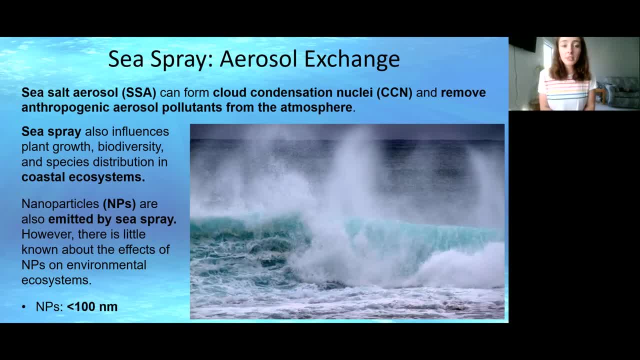 cool, And sea spray also influences plant growth, biodiversity and species distribution along coastal ecosystems. So as waves crash into a coastal area, sea spray containing salt and nutrients is emitted from those waves. It can be blown by wind, because these particles are really 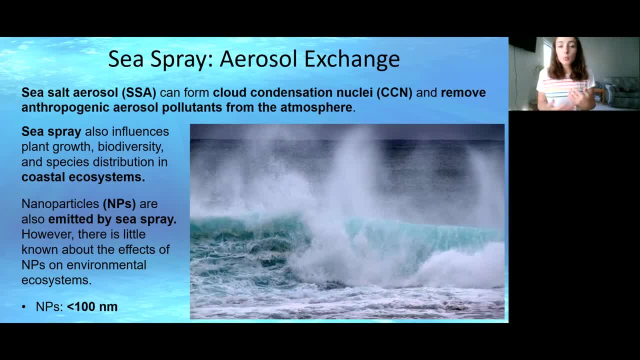 fine and blown into the coast and cause more biodiversity and increased species distribution. due to all these nutrients blowing onto land And, like I said, nanoparticles can also be emitted. However, there is a lot of future research that needs to be done on nanoparticle emission from sea sprays and their distribution in natural. 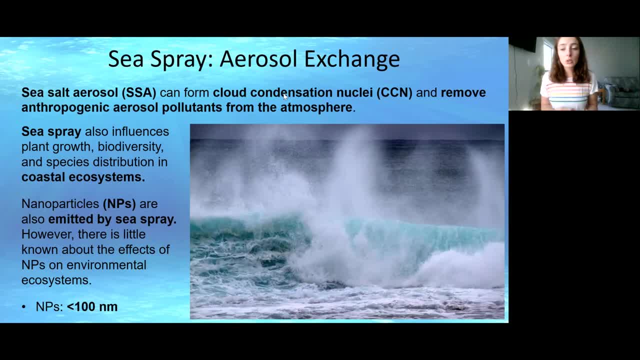 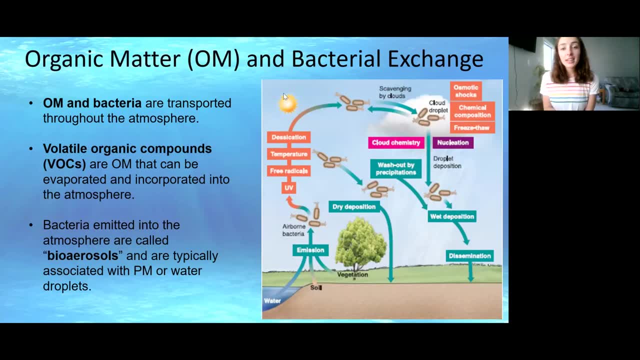 environmental systems, because this is kind of a new area of study. So if you want to do that, you should go into that. It's really awesome and it's really needed. Okay, so last thing is organic matter, or OM, and bacterial exchange from atmosphere to ocean. So this is kind of cool. 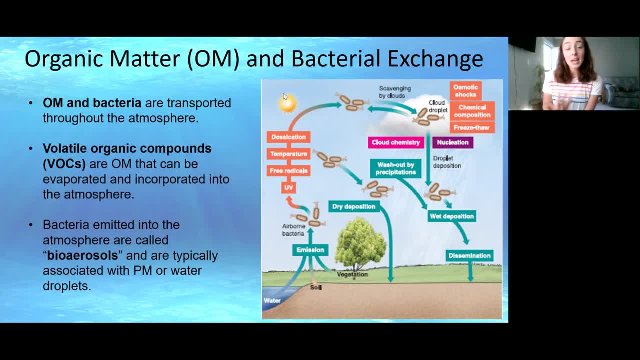 because you might not think that bacteria are in the atmosphere, but they can be, And organic matter actually is as well, although organic matter is a little easier to believe, because organic compounds can be volatile, meaning they can be evaporated or become a gas and be distributed. 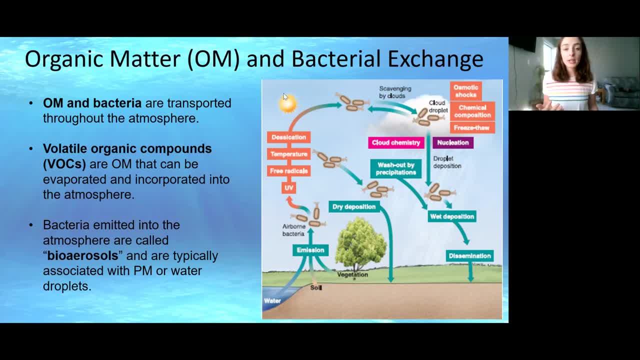 throughout the atmosphere and also be incorporated or associated with particulate matter throughout the atmosphere, And so they're distributed relatively easily. Bacteria, however, have to be accumulated onto particulate matter in order to be distributed throughout the atmosphere, as they are solid, And so they have to be on or part of particles, And so, when they are, they're called. 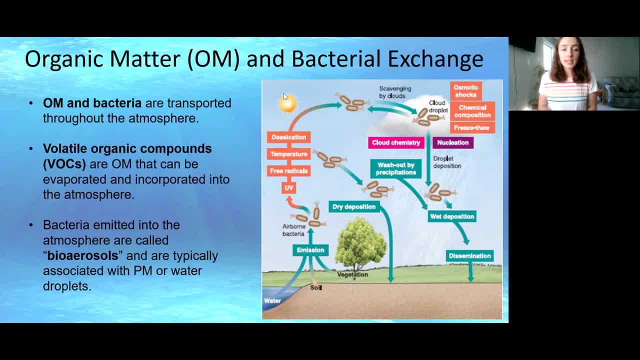 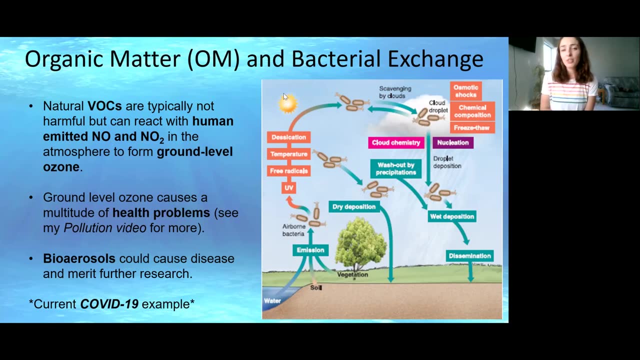 bioaerosols. So in terms of what volatile organic compounds, or organic matter in the atmosphere, and bioaerosols means for our atmosphere and our health and our environment. basically, volatile organic compounds can be natural and are typically not harmful to us, except for the fact that now 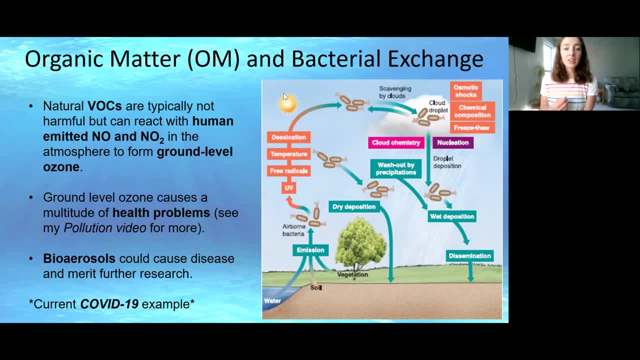 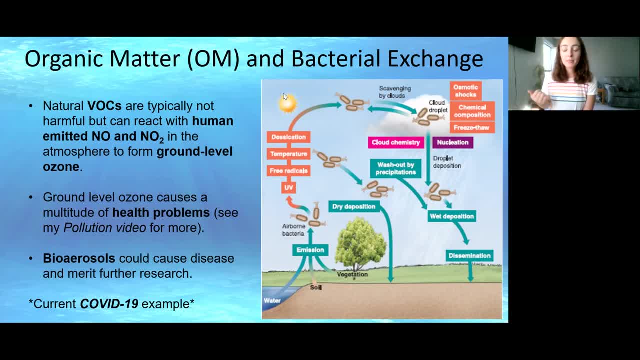 it's not a good thing. Ozone up in the stratosphere is great, but down here in the troposphere is not good for us and can cause very bad health problems. And in terms of bioaerosols, all I could find on this really is that they could cause disease, but they merit further research. 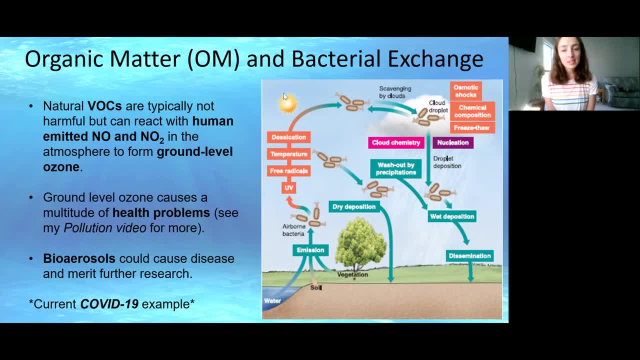 because really not much is known about atmospheric bacteria. Go figure, I think it's a really cool area of research. If you want to go into it, I think you totally should. I think it will have huge implications for our future and be very important. One thing I did: 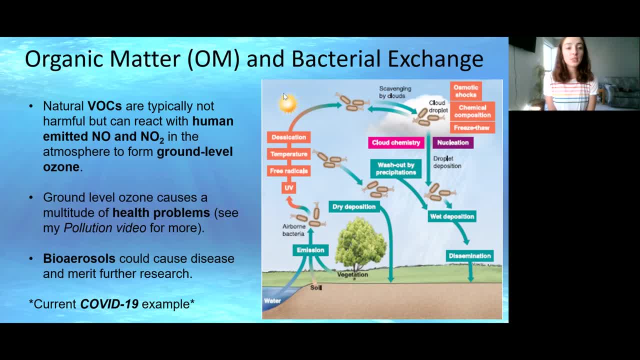 but down here is current COVID-19 example to remind myself to discuss viruses. Viruses are also important. They're not necessarily bacteria, but they are technically bioaerosols because they're bio. Well, I guess this can be disputed whether viruses are life or not, but I think 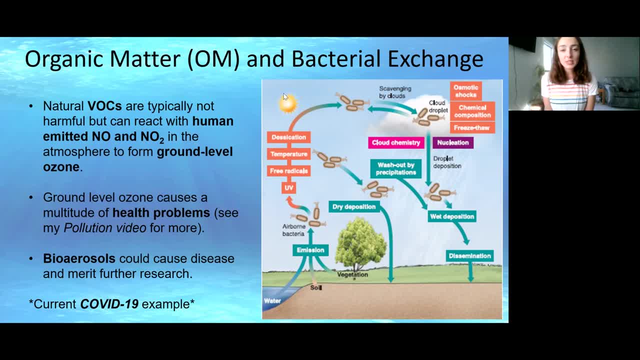 they're technically under the category of biology in terms of study. So yeah, viruses also can be aerosols, and harmful aerosols at that, because obviously we know that viruses can cause crazy epidemics, Pandemics, and it's just not good. And right now we're going through COVID-19, which is the reason. 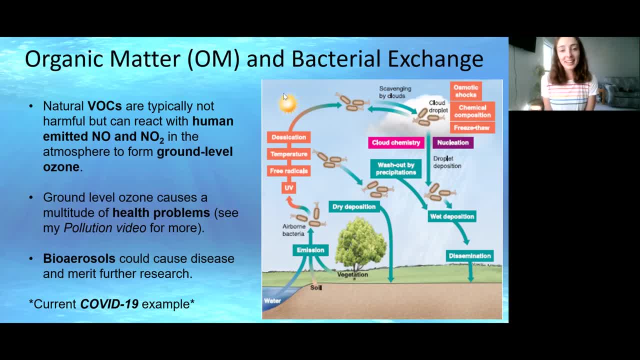 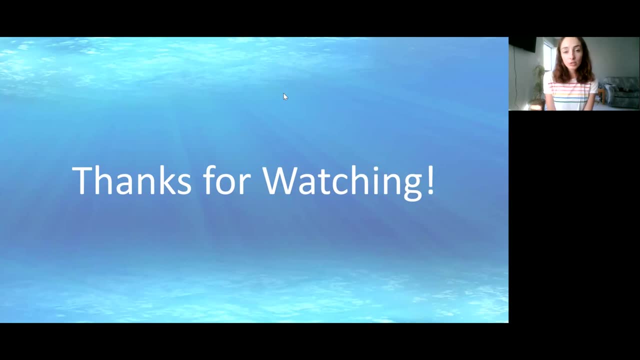 I started this channel because I'm home, I'm bored, But I also want to try and help you guys understand concepts that I find are not available on YouTube as much as they probably should be. So with that, I hope that this was helpful. I hope you learned something about how the ocean